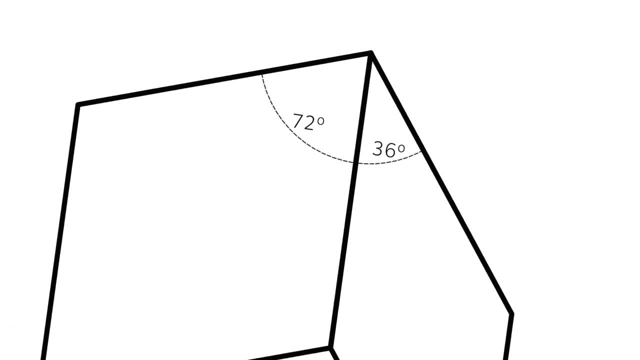 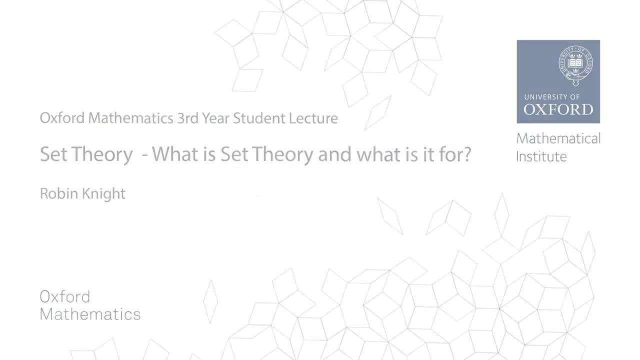 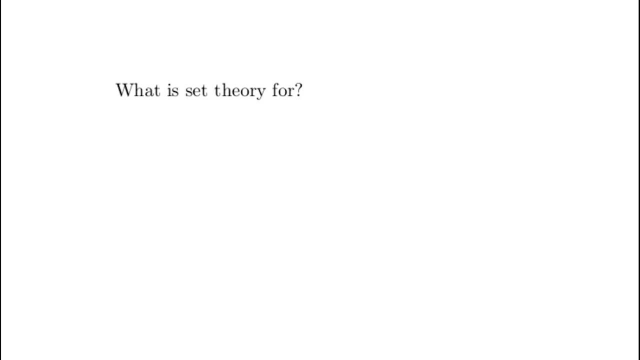 What is set theory for? In other words, why am I spending so many hours of my life lecturing about it? Why are you spending so many of your hours listening to the lectures? Why bother with set theory? Well, this is an answer that you may have very well have originally decided the answer to. 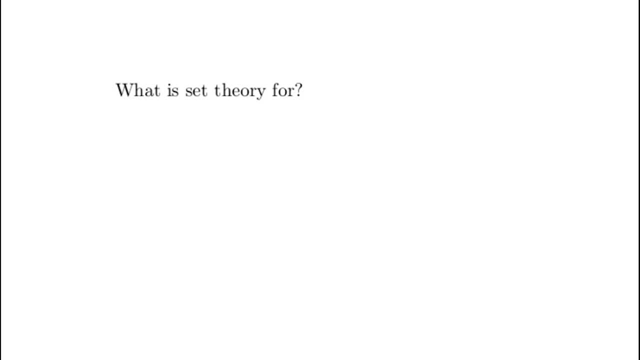 for you. I'll say what my answers to this question are. Set theory is one of those bits of mathematics that some people- but not, though very far from everybody some people- have already met before they went to university. I was one. So at our primary school they taught us some basic set theory intersections. 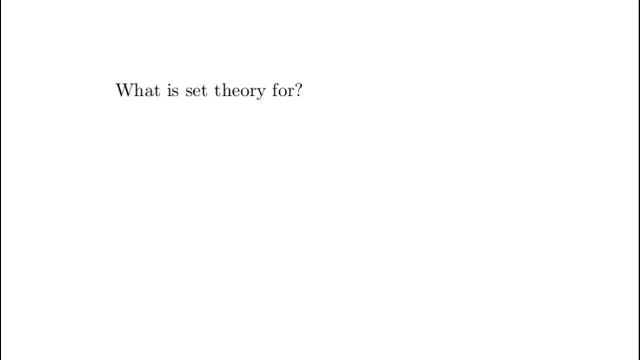 unions, that kind of thing. It was trendy for a while. I thought at the time: you know what on earth is this all about At that level? set theory was just a way of thinking about logic. There's a lot more to it. When I was a bit older, my father told me about 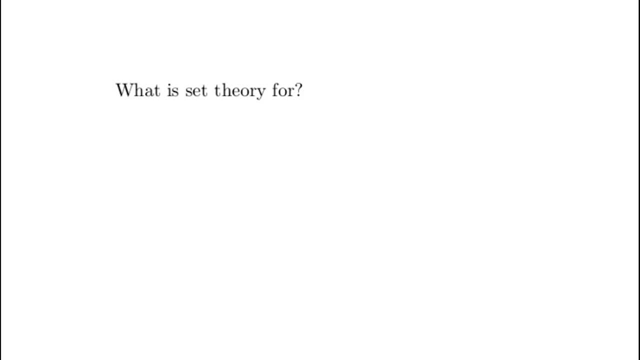 infinity and about how to do arithmetic with infinities, And I thought that was amazing And that is going to happen in this course. Anyway, what is set theory for? And if you haven't met it before, then perhaps you've heard about its philosophical ramifications, about the paradoxes. 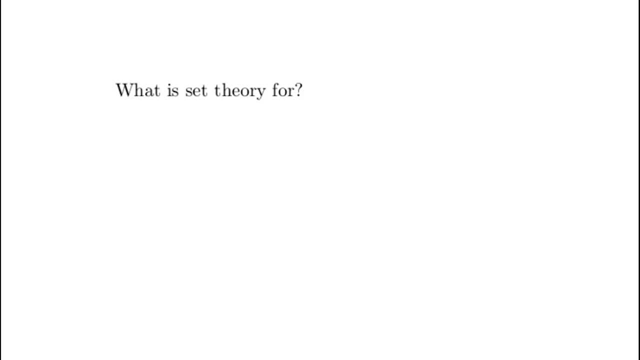 of set theory, about the ways you can use set theory to establish mathematics. I'll talk about some of those things as well. Anyway, what is set theory for Historically? the answer is that Cantor originally developed it for proving a theorem about Fourier. 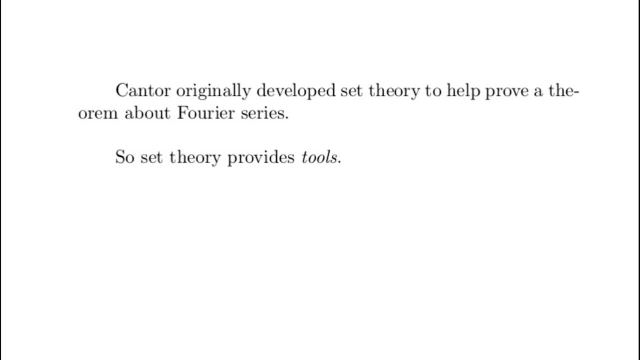 series. So you try and express a function as a sum of cosines and sines. Sometimes it works, sometimes it doesn't. The theorem that Cantor proved- Actually it wasn't the so much the theorems itself, He had a set of theorems. He actually had an infinite transfinite series. 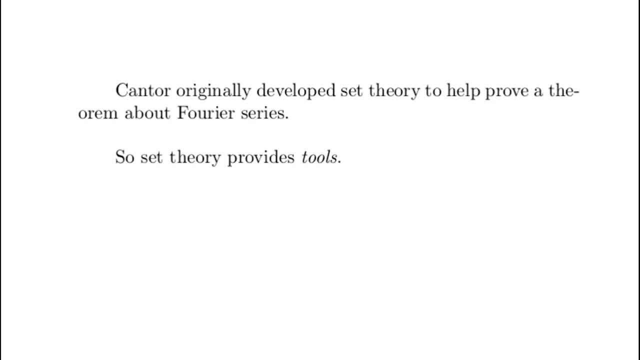 sequence of theorems and he needed to talk about that infinite, finite sequence. he ended up inventing set theory to do it. Set theory then provides tools. they provided the tool that Cantor needed on that occasion. they provide it provides other tools as well. So cardinal numbers, Cantor. 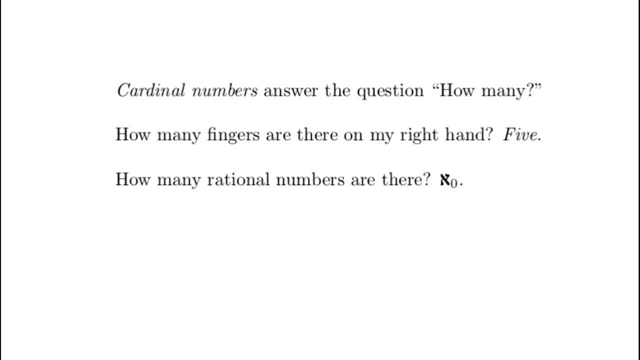 discovered these. a cardinal number answers the question: how many? The word cardinal comes from the latin word for a hinge, so a cardinal. cardinal numbers are the pivotal numbers, the numbers that everything else turns on, so the most important numbers. Okay, so cardinal numbers answer the question: how many. How many fingers are there on my right hand? There are five. 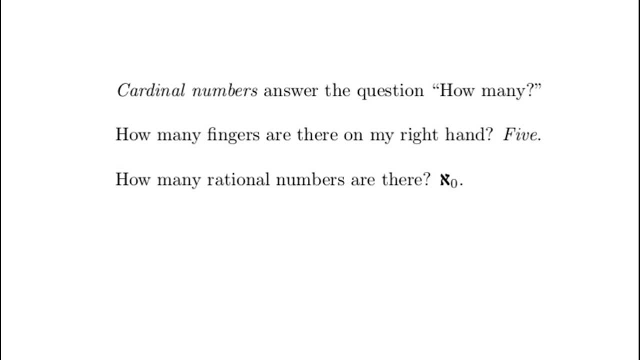 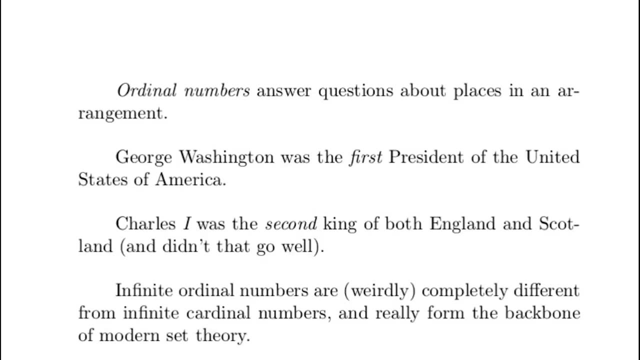 How many rational numbers are there? I'll have zero, Okay. ordinal numbers. ordinal numbers answer a different kind of question. they answer a question about places in an arrangement, and in English and in many other languages there are special words to refer to ordinal numbers. so George Washington was the first president of the United States of America. Charles I was the. 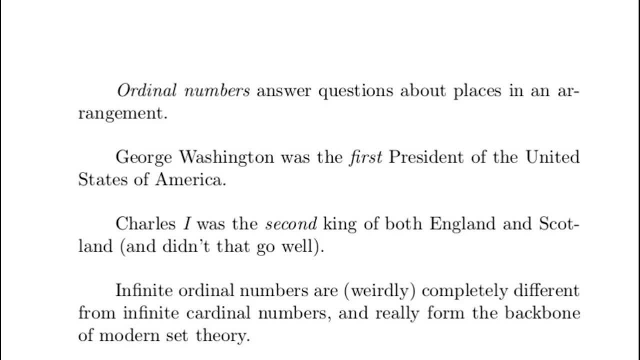 second king of both England and Scotland and so far the only king of England to be executed for treason. the infinite ordinal numbers. Now, the infinite ordinal numbers are weird. The thing that's most weird about them is that they don't correspond neatly to the infinite cardinal. 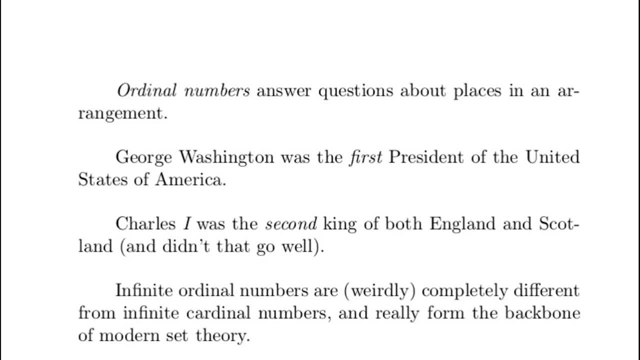 numbers in the way that the finite ones do. OkayThe ordinal numbers are set. theorists refer to them all the time. The ordinal numbers, okay, set theorists refer to them all the time The ordinal numbers lead to each other. that is that and uh. 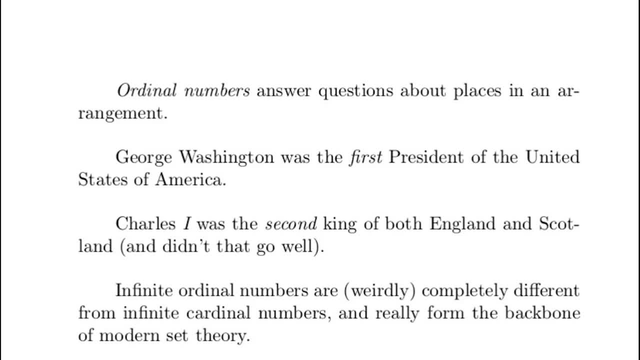 okay. so how many? Very few be one, roguuby, Yes, are the backbone of modern set theory. You hardly hear a set theorist opening their mouths without mentioning an ordinal number. I exaggerate, but not much, Okay. so set theory provides tools, and set theorists are also very good at. 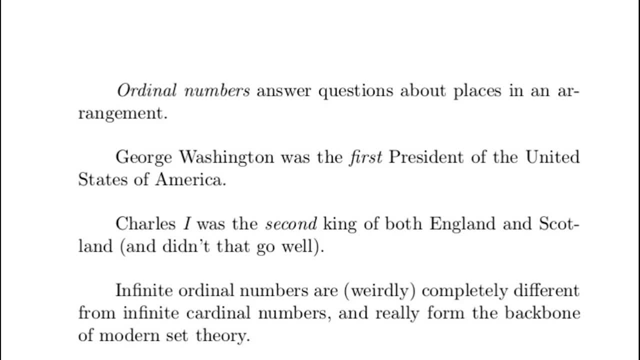 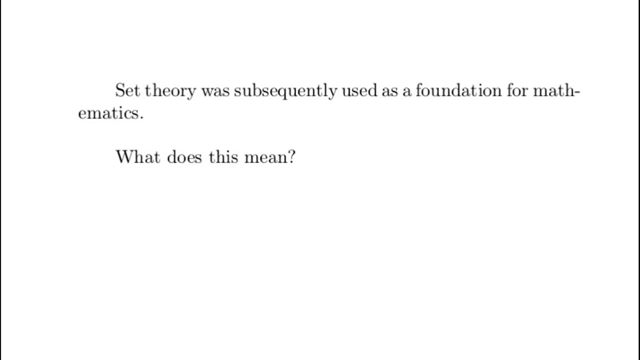 doing schemes of coding, so representing sort of coding up structures in various kinds of data structures. Yeah well, we won't be doing so much of that this term we'll certainly be seeing the cardinal and ordinal numbers. Okay, later on, a few decades later, set theory was developed as a foundation of mathematics. and if 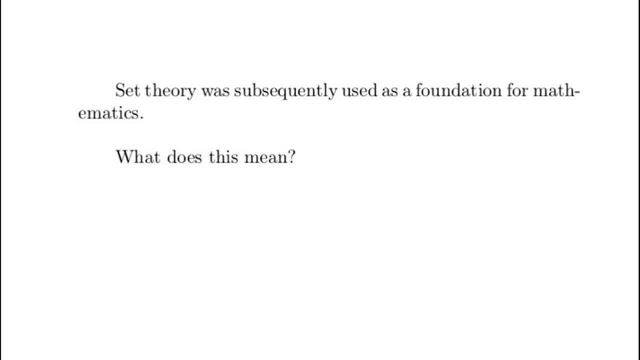 you're into the philosophy of set theory. this may very well be what you're interested in, But what does it mean to say that set theory can be a foundation for mathematics? Well, the metaphor is from building. So when you build a house before you, 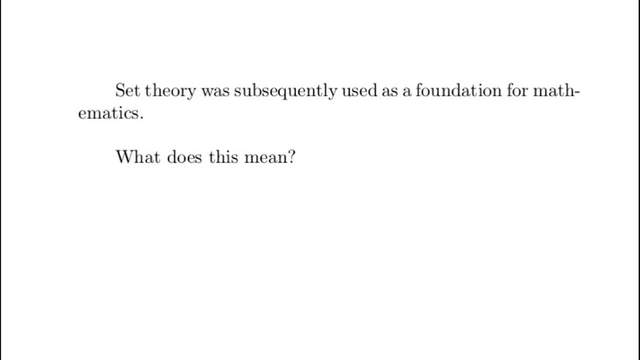 actually start building the house itself. you dig down into the ground and set a foundation so the house won't fall over. So, presumably, set theory is supposed to be something secure and solid underground that we can build the building of mathematics on top of. Well, how does that work? Well, the first thing. 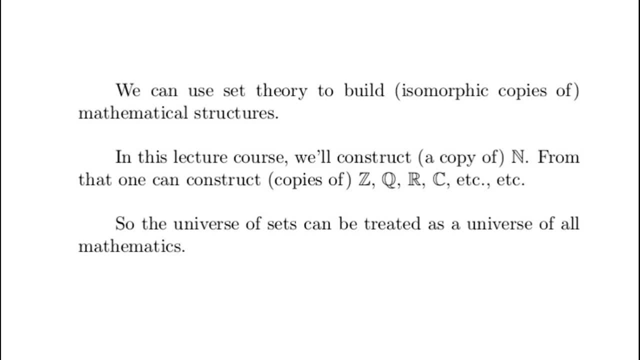 i is that in set theory we can make copies of a lot of mathematical structures. so in this lecture course we'll construct the natural numbers. so the natural numbers are not basic to mathematics anymore. they can be defined in terms of something simpler, namely sets. and once you've got the 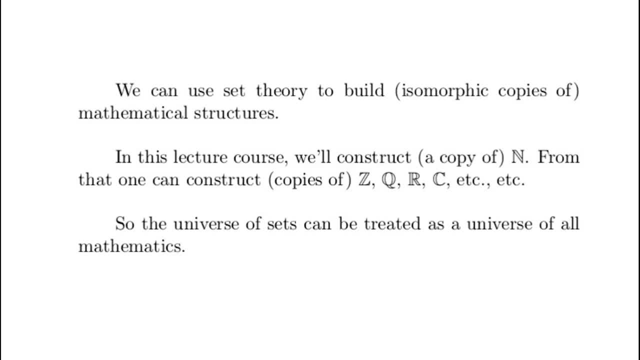 natural numbers we can construct the integers, the rationals, the reals, the complex numbers and all of those that the constructing z, q and r from n is not on the syllabus. i'll say later on in the course in a handout how that's done. so that means that the universal sets can be treated as if it was. 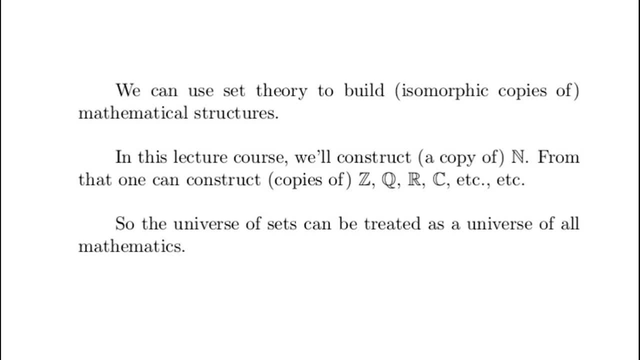 the universe of all mathematics. so we can represent the natural numbers by a set, we can represent q by a set, and so on. and so we can say: okay, when we're doing mathematics, the universe of sets is it, it's everything, and we ignore everything else. okay, so that's one way in which set theory is a foundation, for mathematics is an. 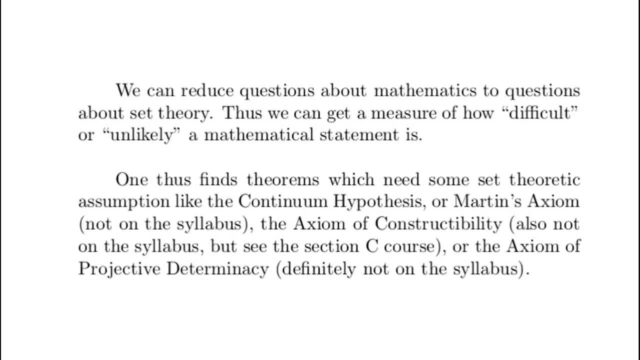 ontological way, if you like. the other question is about provability. so, um, we, we might have a complicated mathematical question. uh, we can sometimes reduce it to a set theory. but we can also reduce it to a question about set theory. so, um, uh, so we, we, we try and prove our. 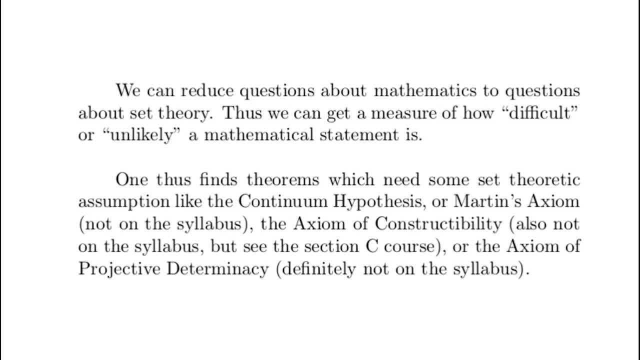 theorem. we might find that our theorem proves really- uh, proves itself really easily using only very basic set theoretic assumptions. we might find that it's really sophisticated and fiddly and uses very complicated and powerful set theoretic assumptions. so we get a measure of how difficult a mathematical statement is, or, uh, if the set theory is really complicated. 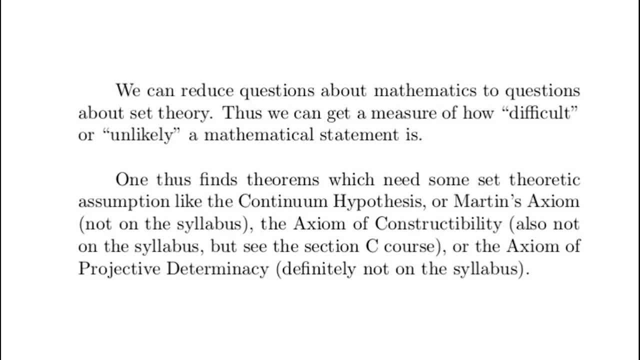 theoretic axiom we need is a bit unlikely how unlikely our statement is so um, so there are. we have set extra set theoretic axioms. i've mentioned a few: the continuum hypothesis, martin's axiom, the excellent constructability, the axiom projective determinacy- uh, projective determinacy. 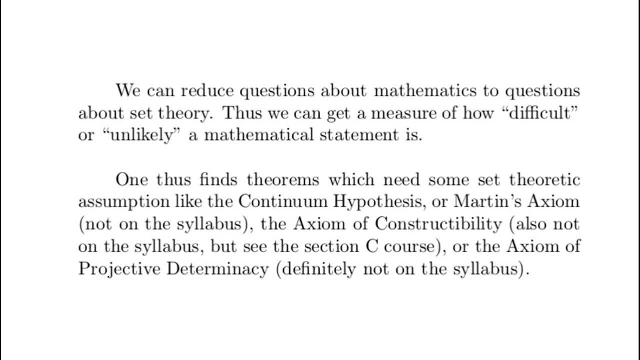 is particularly powerful or, if you like, unlikely. okay, so, um, we get the. i mean so, um, very often, in certain areas of mathematics, we keep track of which set theoretic axioms we need to prove our mathematical results, and our list of set theoretic axioms provides a uniform scale of. 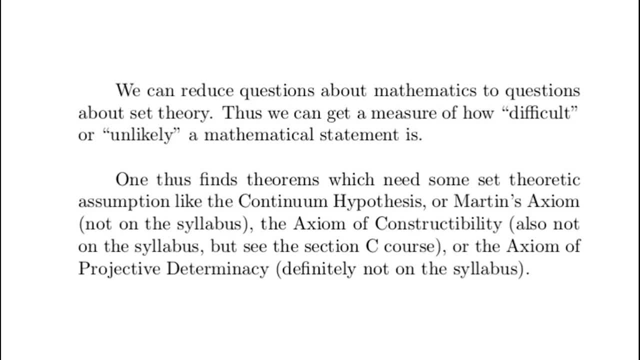 sophistication anyway. so so, um, that's an epistemological, um way in which, uh, set theory could be a foundation of mathematics, a way of saying: you know, how do we know that something is true? or we can prove it if we make the following assumptions: anyway, so that set theory is a foundation for mathematics. 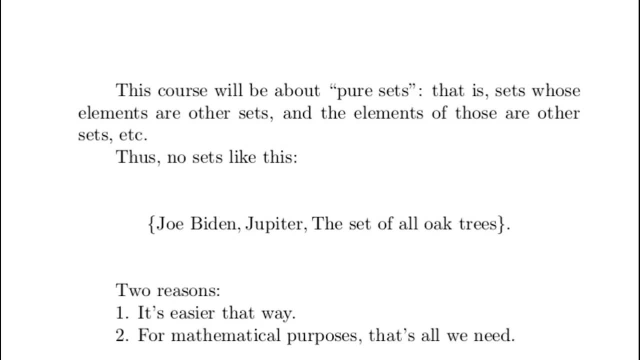 um and um. i should say that when i talk about the universe of sets, i'm talking about pure sets, so sets whose elements are other sets, and so any any set that i'm talking about in this course will be, if you like, a bunch of curly brackets arranged in a row, and there'll be when we uh dig down through the pairs of curly brackets.